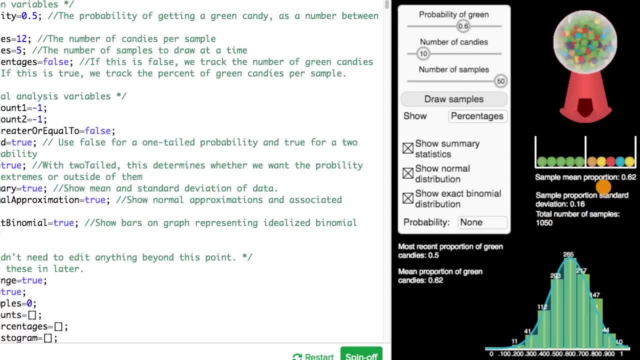 is that it's a very large sample And what's interesting here is we're seeing experimentally that our sample, the mean of our sample proportion here, is 0.62.. What we calculated a few minutes ago was that it should be 0.6.. 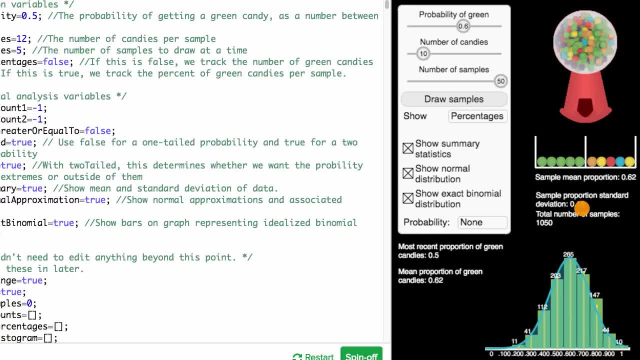 We also see that the standard deviation of our sample proportion is 0.16.. And what we calculated was approximately 0.15.. And as we draw more and more samples, we should get even closer and closer to those values. And we see that for the most part. 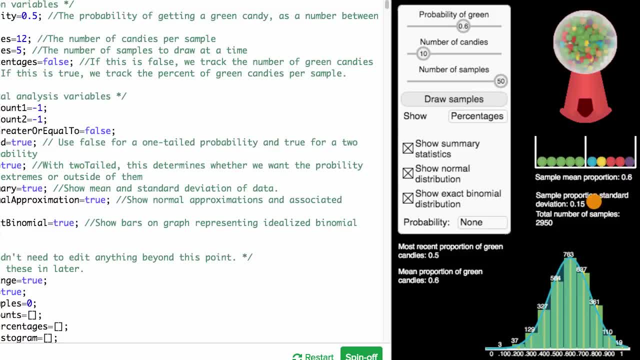 we are getting closer and closer. In fact, now that it's rounded, we're at exactly those values that we had calculated before. Now, one interesting thing to observe is when your population proportion is not too close to zero and not too close to one. 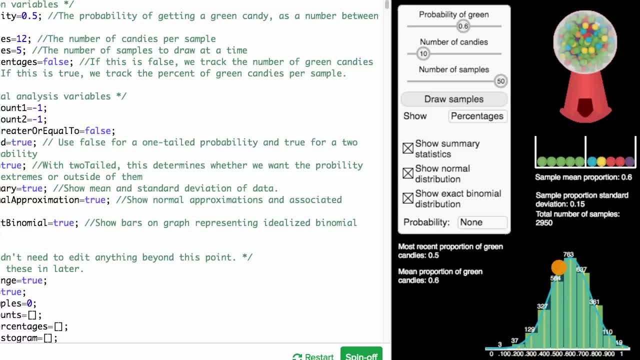 this looks pretty close to a normal distribution And that makes sense because we saw the relation between the sampling distribution of the sample proportion and a binomial random variable. But what if our population proportion is closer to zero? So let's say our population proportion is 10%- 0.1. 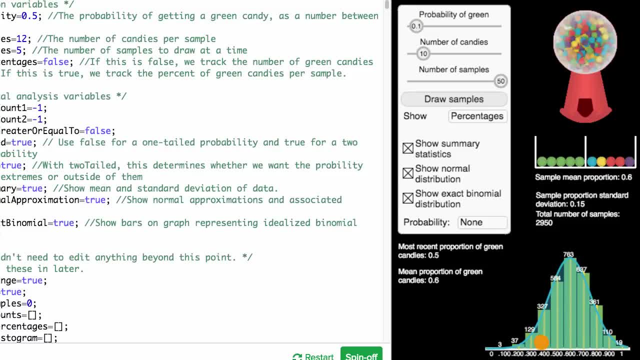 What do you think the distribution is going to look like then? Well, we know that the mean of our sampling distribution is going to be 10%, And so you can imagine that the distribution is going to be right skewed. But let's actually see that. 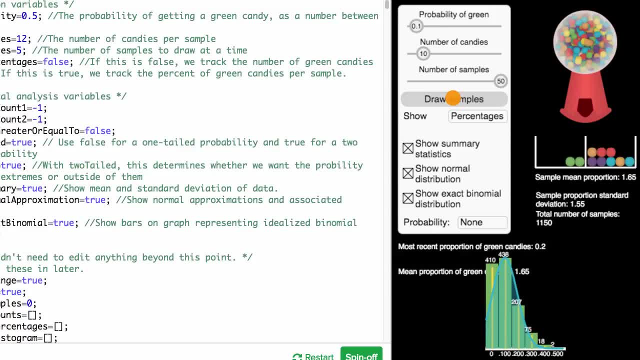 So here we see that our distribution is indeed right skewed, And that makes sense, because you can only get values from zero to one, And if your mean is closer to zero, then you're gonna see the meet of your distribution here, and then you're gonna see a long tail to the right. 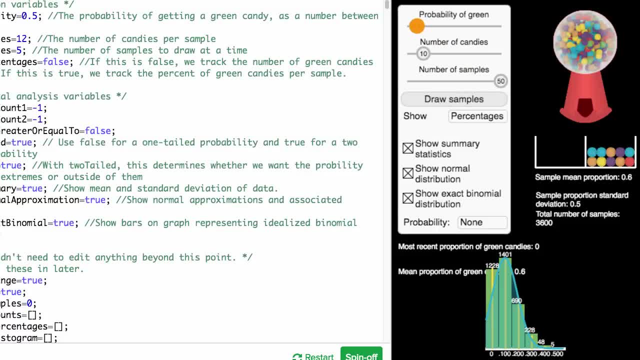 which creates that right skew. And if your population proportion was close to one, well, you can imagine the opposite's going to happen. You're going to end up with a left skew, And we indeed see right over here a left skew. Now, the other interesting thing to appreciate is that 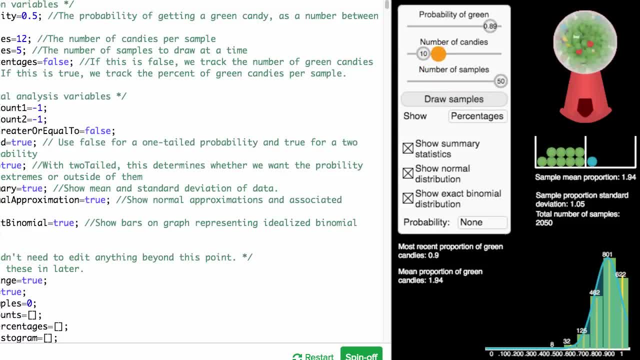 Now, the other interesting thing to appreciate is that. Now, the other interesting thing to appreciate is that the larger your samples, the smaller the standard deviation, And so let's do a population proportion that is right in between. And so here this is similar to what we saw before.